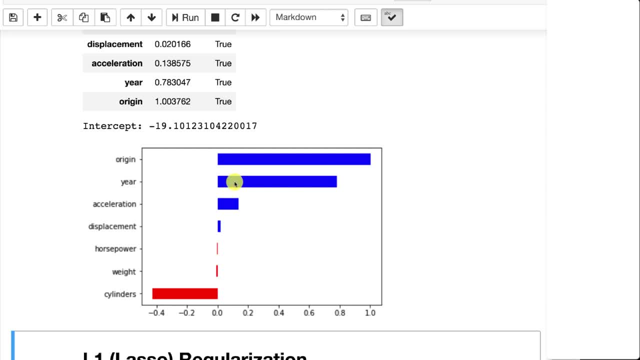 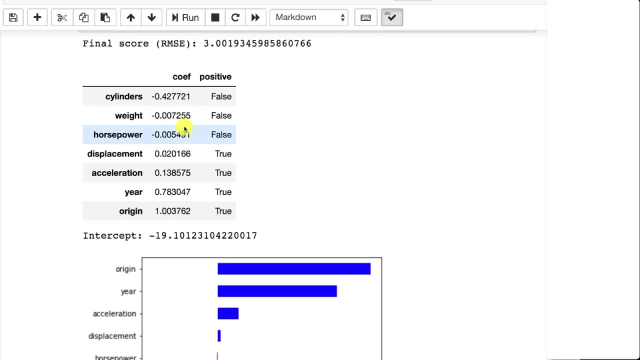 Year also is important, because as the year increases the cars got more efficient And you can actually see the values, So you could truly calculate a car's miles per gallon. You just take all of these values, multiply each by the coefficients, and then you add in the intercept And it'll give you a rough estimate of. 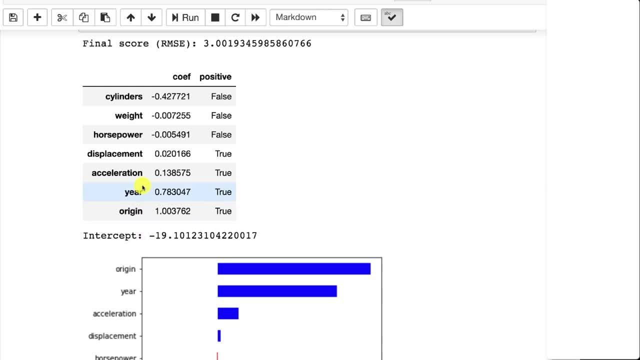 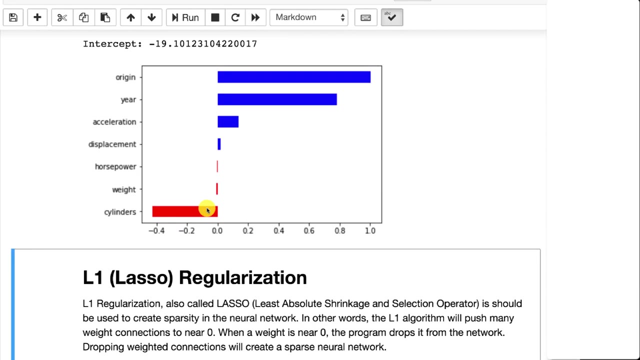 of what the miles per gallon is. By the way, I will point out too that origin. I probably should have been turning that into dummy variables, but here we're just treating it as a basic numeric. I've never found that to give me much, much lift on this particular one. Let's look at Elwan Lasso. Elwan Lasso makes use of 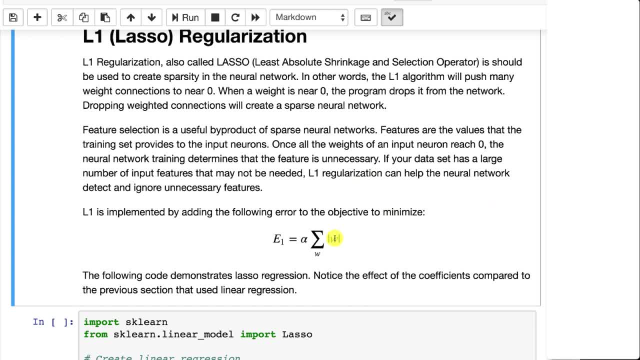 We're basically adding the weights together, So we're summing the weights and using the weights as a penalty. so if the weights get too high, the absolute value of the weights gets too high. that counts along with the error, so the difference between the expected outputs and 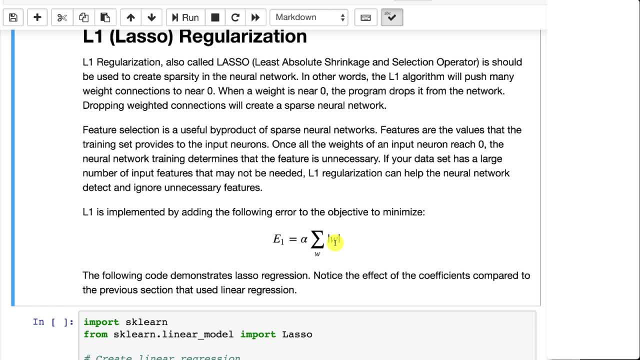 the real outputs and those two together. you're giving the neural network multiple objectives, as it's trained. you're saying, okay, on one hand, be as accurate as possible, but on the other hand, don't let those weights get too big. and this deals somewhat with Occam's razor, in that the 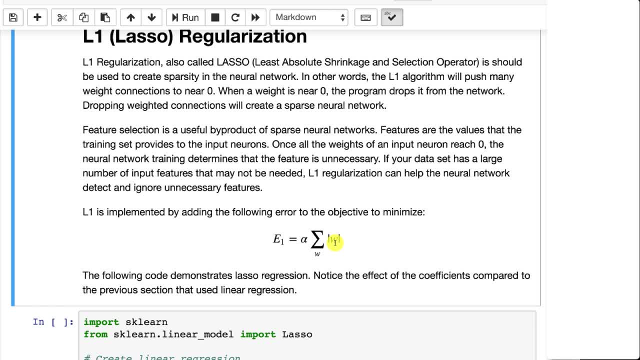 more simple solution is usually the better one. now, the absolute value is a fairly sharp cutoff, so that will tend to completely eliminate some inputs. this is good for feature selection l1 if you have a lot of input features and you are thinking that some of those are not necessary. 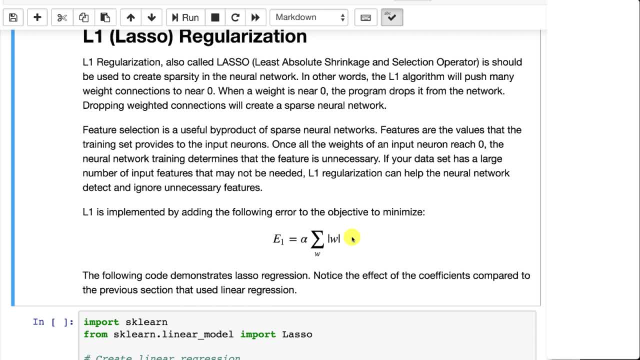 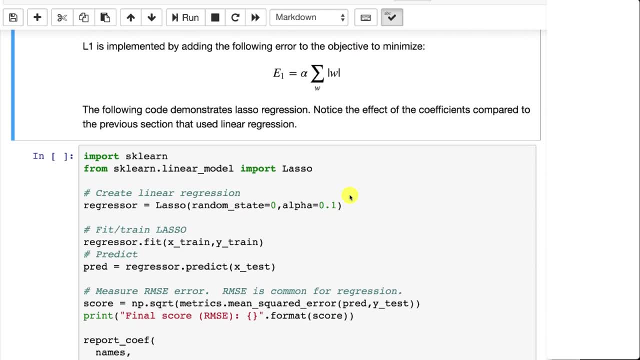 l1 can be a good regularization technique because it simply cuts them out and lets the neural network- later neural network, for now linear regression- focus on the more important ones. we'll go ahead and run this one. you can see that it cut off a lot of these down here. it pushed them. 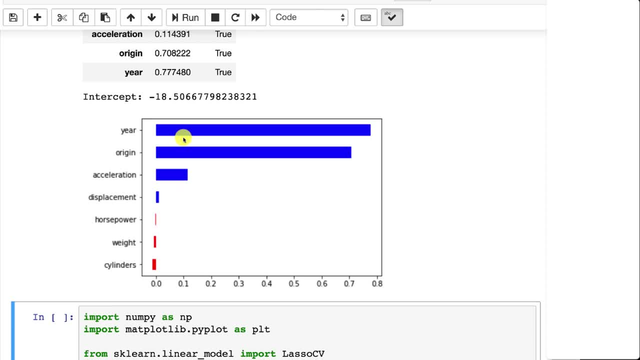 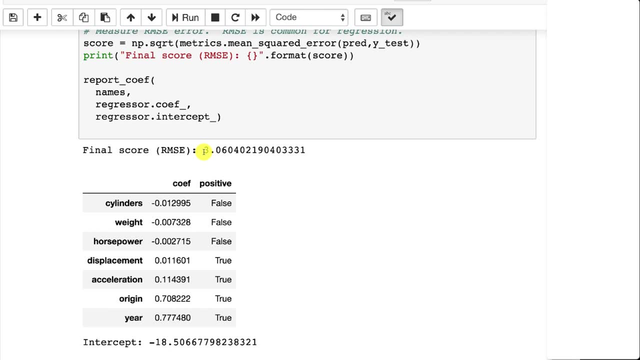 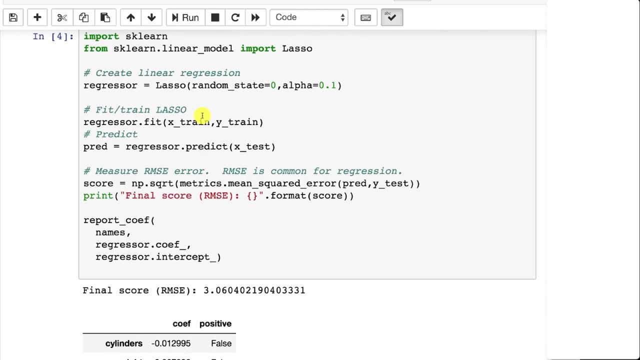 to near zero and we're focusing just on year and origin. you can also see the final score is is not that bad, considering that we are not using the full, the full data set, the full columns of the data set. these are getting pretty much eliminated. by the way, you'll also notice that we specified 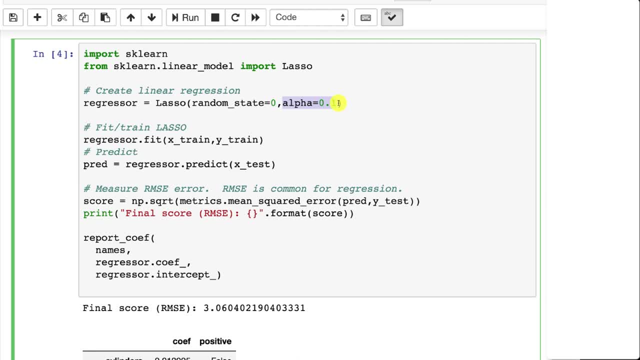 a alpha. that is, the degree to which the weights are counted as as a bad indicator for, for the multi-objective. so you're giving it two objectives. whenever my boss comes to me and says, okay, this is a high priority and this is a high priority, okay, you've got a weighted, which which of those two high priorities is the highest high? 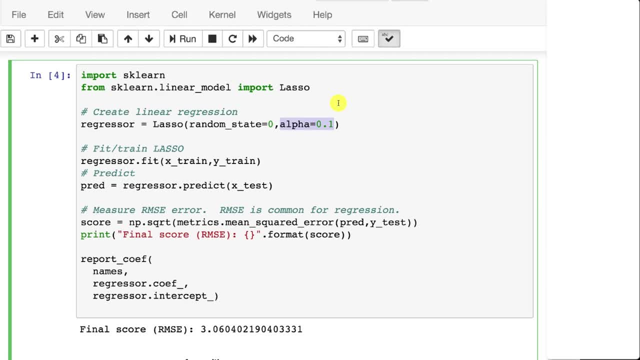 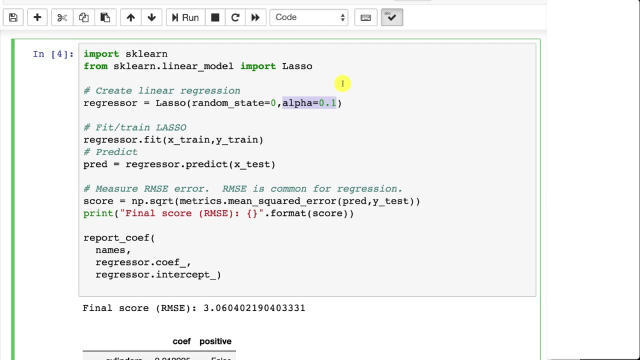 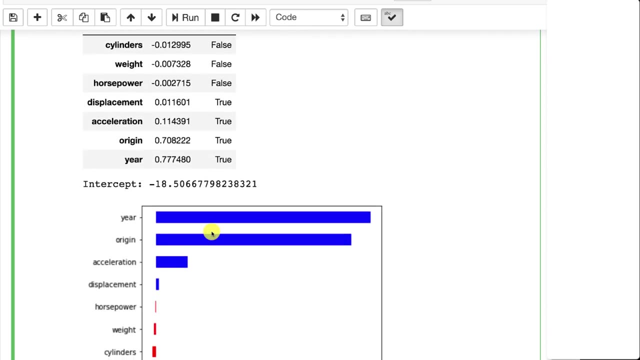 priority and this is what's going on there. the this is very much telling the neural network that, okay, yes, the regress, the regularization is important, but it's only one tenth as important as getting an accurate result. but nonetheless, this this gets it to chopping off some of those, so it's it's pretty effective. it is. 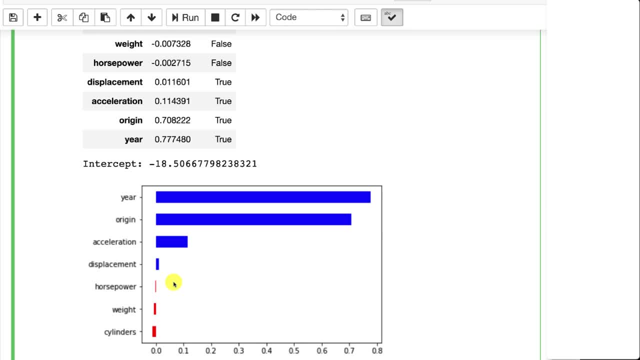 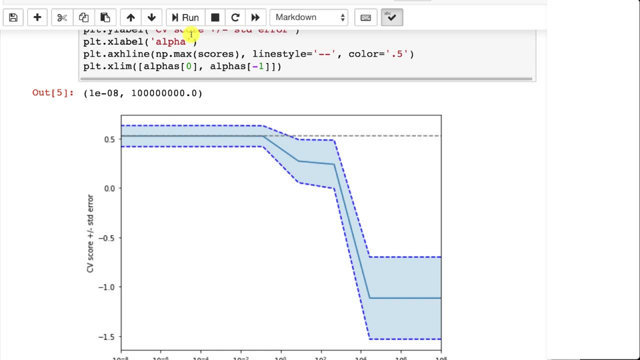 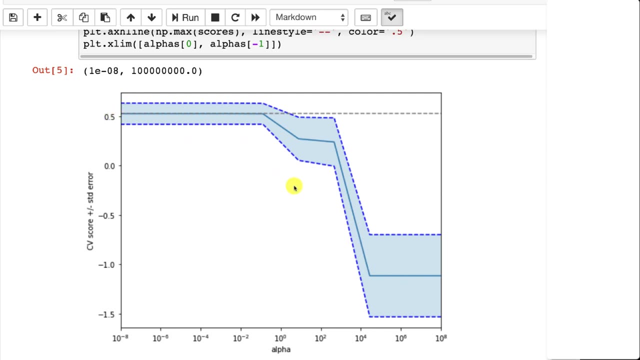 it is doing what a lasso you're expecting it to do. it is removing unneeded columns. now what's the effect of changing that? that alpha? you can see, as you make alpha bigger and bigger, the error gets considerably worse. so that's basically what that is is demonstrating. so you don't want to make the 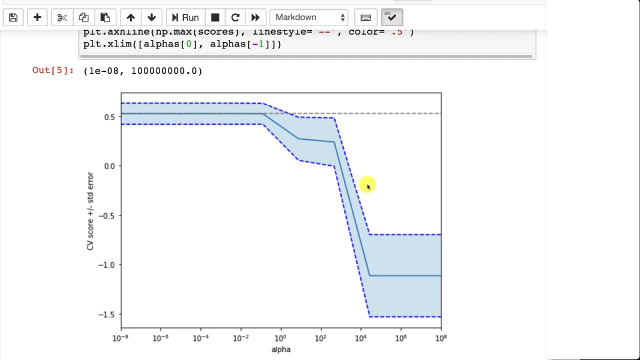 alpha usually too big, but it is. it's yet another hyper parameter to tune. so later when we get to the kaggle competition module, we're going to see how several ways that we can optimize all these hyper parameters, because this is getting to be a lot of things to manage on a neural network. you 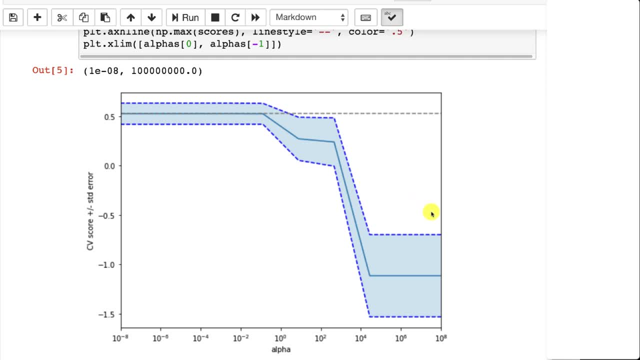 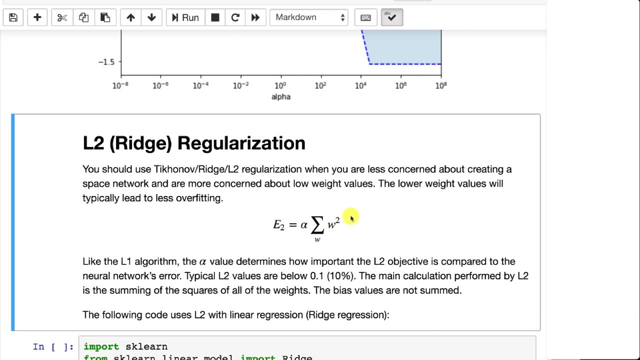 have regularization? how do you pick how many neurons, how many layers? all that kind of l2 ridge regression? instead of taking an absolute value, you're squaring it and that makes it more more rounded. so that causes it to be less harsh on trying to eliminate individual columns altogether and rather just seeks to keep the. 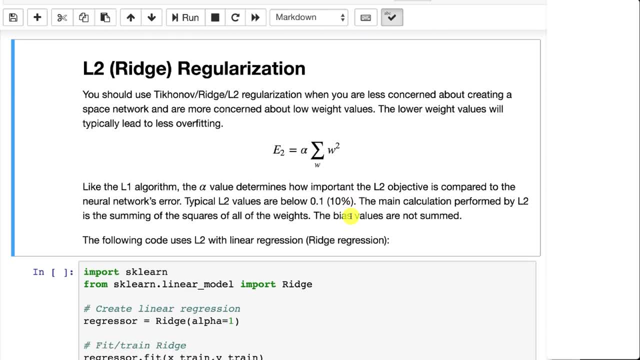 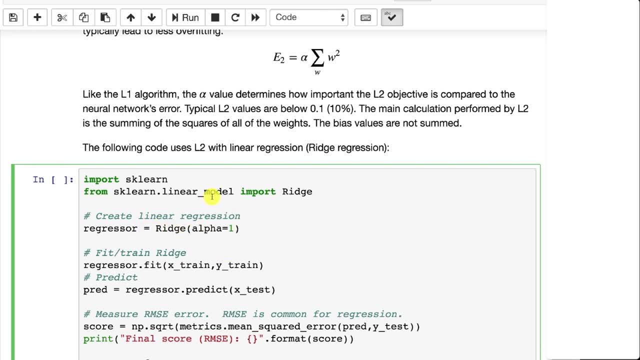 weights down or the coefficients down. this is l2 regression. we'll go ahead and run it. we're using ridge from scikit-learn here. i'm setting the alpha fairly aggressively and you can see the results here. it is definitely pushing some of the middle ones and some of the middle ones and some of the